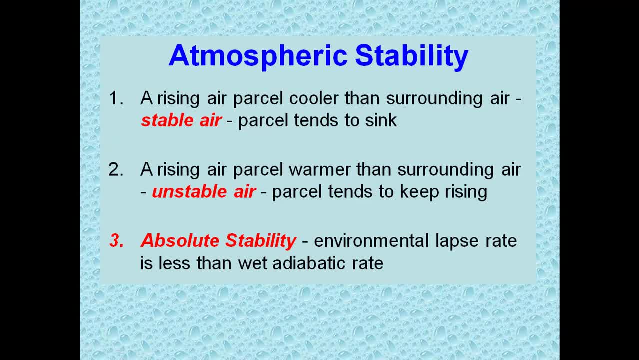 Now we're going to talk about the three different stability types in our atmosphere, and this is very important because if we have an unstable atmosphere, we have air parcels that are willing to rise, and if our atmosphere is unstable and our air parcels are willing to rise, we are causing or creating situations where there can- and oftentimes are, some type of weather. 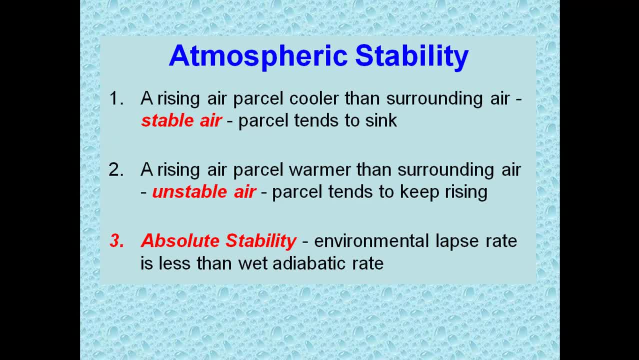 So stable air we talk about when air parcels are willing to sink. So if I took an air parcel and I brought it up at some point in the atmosphere and I released it and it sank back down to its original spot, that is considered a stable atmosphere because air parcels are cooler than their environment. they're cooler than their surrounding environment and thus would want to sink. 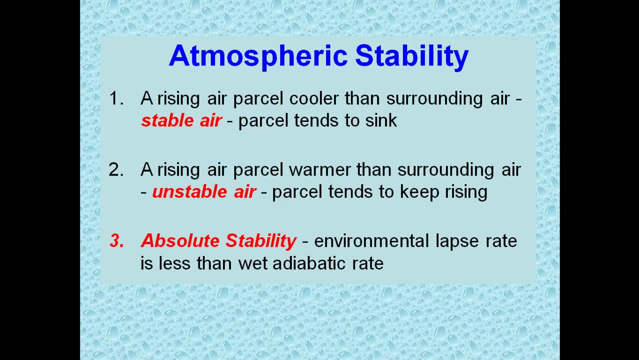 On the opposite side. if I take an air parcel and I lift it up to some point in the atmosphere and it continues to rise, that means that that air parcel is warmer than its environment and is willing to rise and therefore it is going to continue to rise. and that is how you cause weather and that is what an unstable atmosphere is. 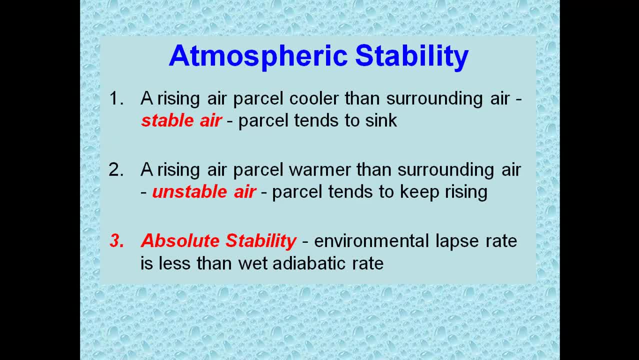 Now you can also have a neutral atmosphere. A neutral atmosphere is just what it sounds like. If I took an air parcel and I forced it to rise and it stood there at the point that I raised it to and it didn't rise anymore or it didn't sink. that's what's called a neutral air parcel. 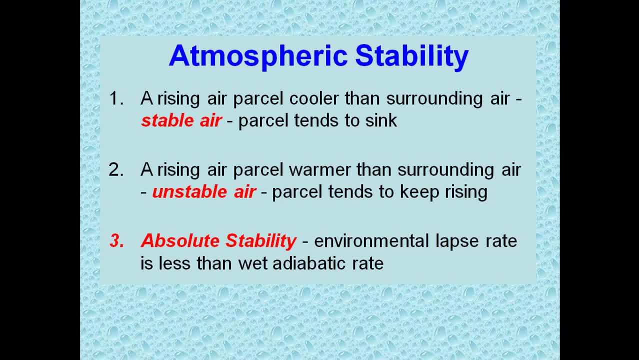 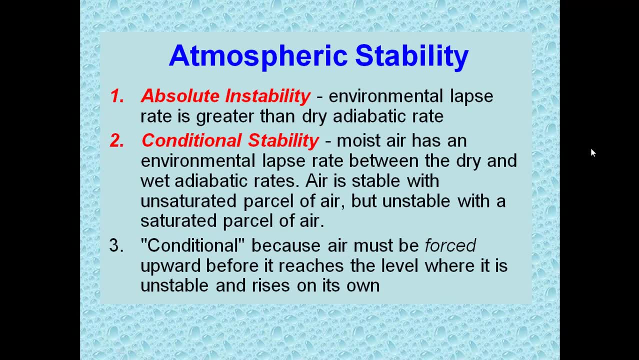 And this is where air parcels could really go either way. Now, based on that idea, we can talk about a couple more stability types, One of them being absolute stability, the other two being absolute instability and the third being conditional stability. So I know, this sounds like a lot, but we're going to break it down. 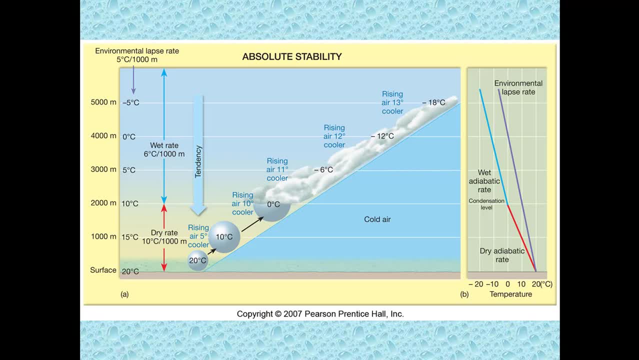 Absolute stability simply means this: you have an air parcel that is cooler than its overall environment, that is comfortable with where it is, but it's forced to rise higher in the atmosphere. but it always would have been better off, or have preferred, it being in the spot where it originally was. 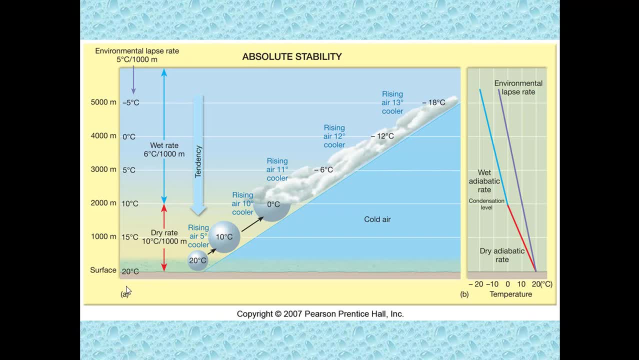 And so in this example here you have some kind of frontal passage. Oftentimes in this situation this is usually some kind of warm front where cooler air is already in place but warmer air is moving into a region. But because cold air is much more dense than warm air, when a warm front moves through, 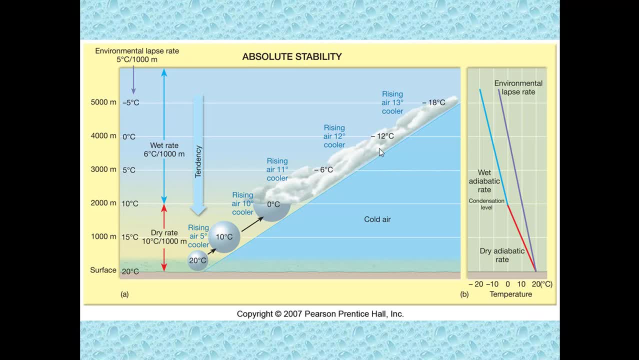 that usually means that warm air has to ride up over the colder air that is already in place, And so warm fronts. we're going to talk a little bit more about that later on in the semester. but warm fronts don't necessarily cause as significant of weather events as cold fronts do. 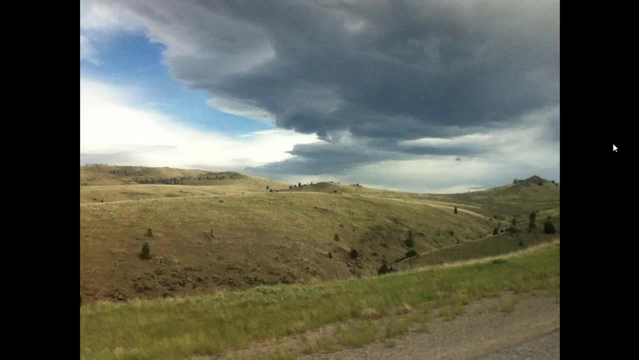 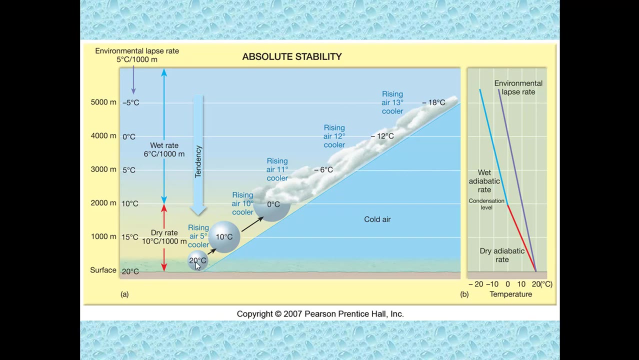 But if you've ever seen clouds that look like this before, this is an example of absolute stability, where the air parcel was comfortable with being either at the surface or at some lower point in the atmosphere, but it was forced to rise over cooler air and it never really wanted to rise in the first place. 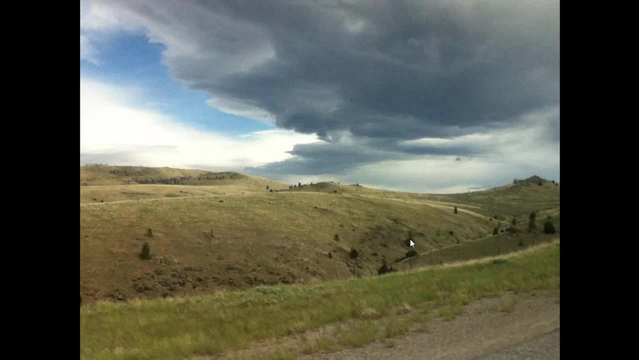 So clouds like this or clouds like this or situations like this here you can see there's a bunch of hilly terrain here, So maybe you had a little bit of orographic lifting. air was being forced to rise over some kind of mountainside. 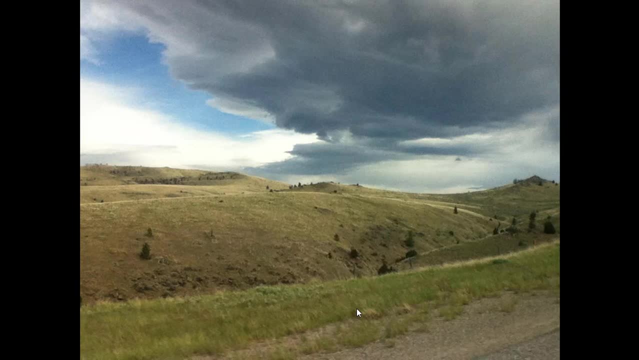 but that air that was already in place was cooler than its surrounding environment. Therefore didn't necessarily want to rise in the first place, but there was enough forcing or enough wind traveling up these mountain ridges or hill ranges that caused this kind of mid-level cloud deck. 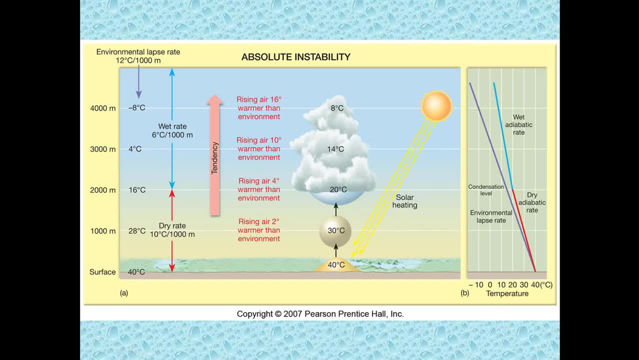 The second type of instability is what we know as absolute instability. Absolute instability is an air parcel that oftentimes is usually neutral. It could go in any which way, but oftentimes when you have an absolute instable atmosphere, it really is due to the sun coming out as solar heating. 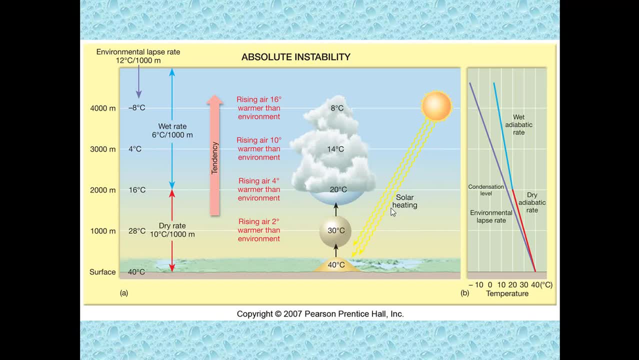 and really just causing the air to rise, causing some localized convective lifting. So the sun comes out, heats the surface of the earth. The surface of the earth heats the air that sits solely near the surface of the earth. It heats by conduction and therefore it becomes warmer than its environment. 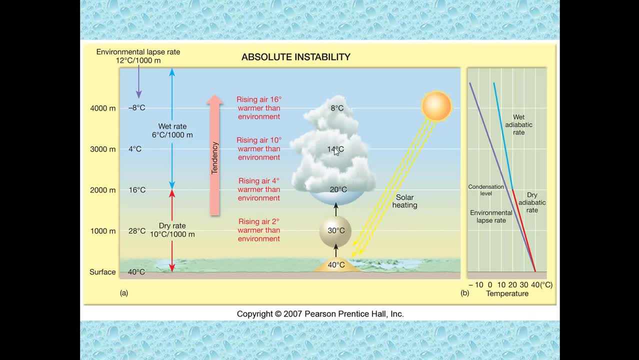 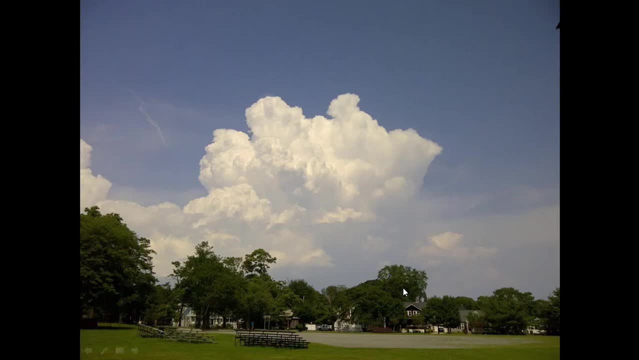 and it rises at the dry adiabatic lapse rate. And so in this case, when you have ever seen clouds like this or like this, you see that the air- and oftentimes these are thunderstorm clouds- the air that was already at the surface was already warm and muggy. 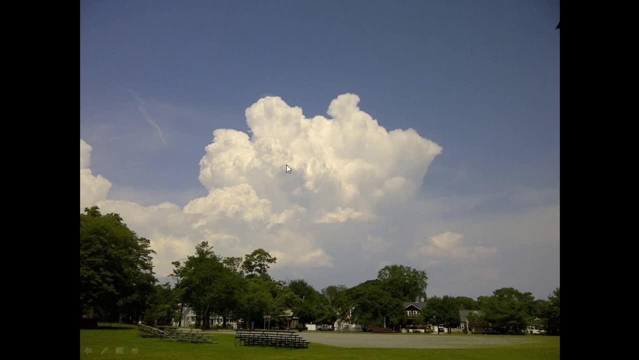 and all it needed was a little bit of push from solar heating to really cause air parcels to start rising higher up in the atmosphere, And probably the height of this cloud roughly is probably anywhere between 10 and 15,000 feet high up in the atmosphere. 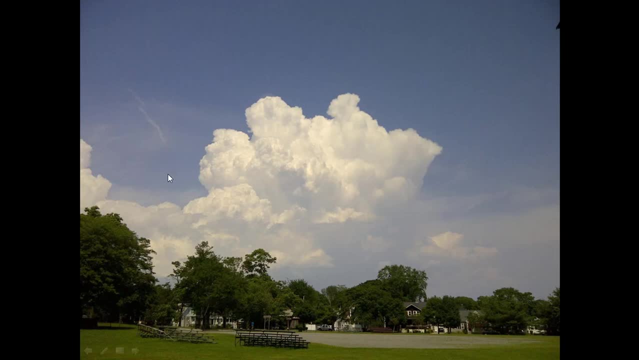 So just to kind of put a little bit of a scale on this, I was actually um having a Frisbee game in the park and I took this picture of it just because it was so beautiful. This was a thunderstorm that was actually being created towards the other part of the town that I live in. 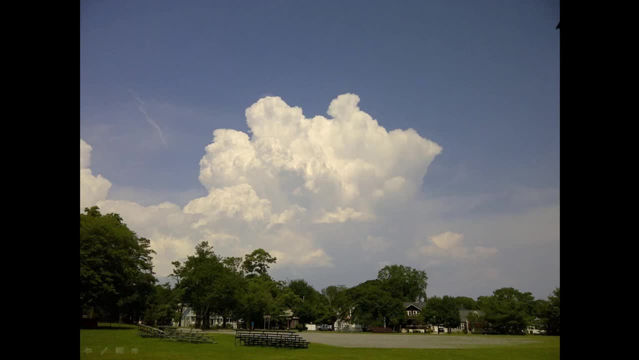 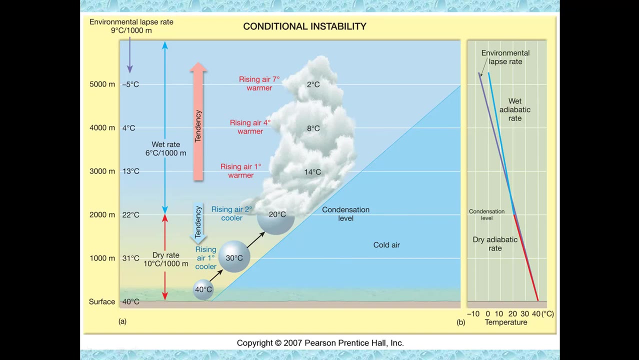 And this was a perfect example of absolute instability. Now, conditional instability is really just a hybrid of the two, And so conditional, as in air parcels- were cooler than their environment and thus they were already stable To begin with. they were happy where they were. 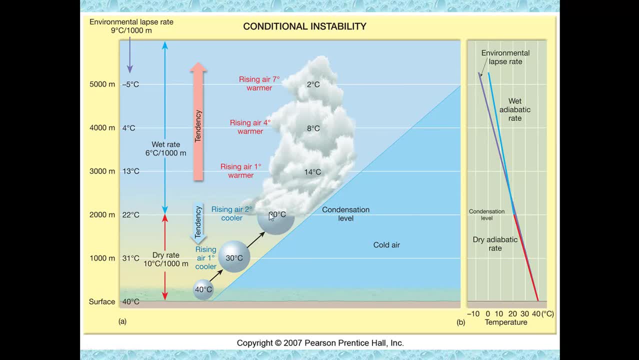 but something forced them to rise. They rose to a certain level in the atmosphere and then actually became warmer than their overall environment and then just kept continuing to rise. So this is a great example of when there is an inversion in place and we have a thunderstorm situation, and we're going to talk a little bit more about that when we talk about thunderstorms. 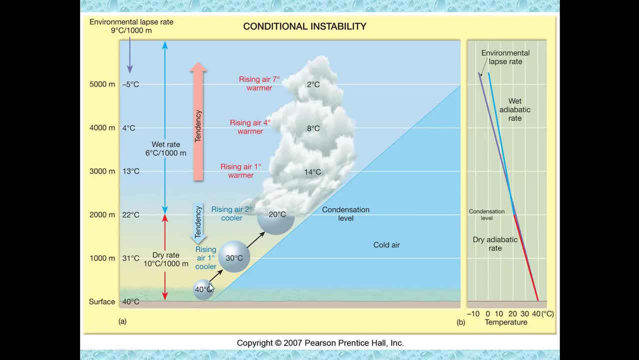 But just in this example here you had an air parcel that was 40 degrees at the surface. It rose at the dry adiabatic lapse rate to a certain point in the atmosphere here, where it basically was equal to its dew point temperature, started making a cloud. 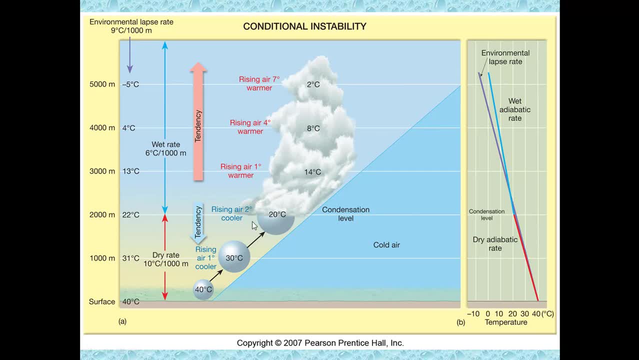 But here you can see, at this level the overall environment was 22 degrees Celsius, but the air parcel was 20 degrees Celsius. So here air parcels were still cooler than their environment. Not by much, but they were still cooler. Something was forcing these air parcels to continue to rise. 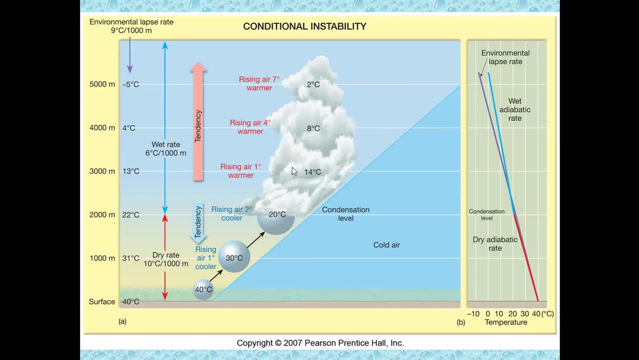 and now at 3,000 meters, or 3 kilometers, the air temperature of this air parcel was now 14 degrees Celsius, but the surrounding air was 13 degrees Celsius, So at this level this air parcel was warmer than the overall environment. 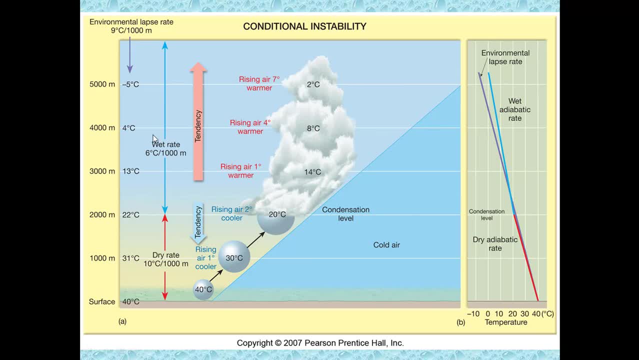 It went up to 4,000 meters And here the air parcel is eight degrees Celsius, but the overall environment environment was four degrees celsius, and so on and so forth. so this is what conditional instability is: it's air that necessarily didn't want to rise in the first place, but got to a certain point that 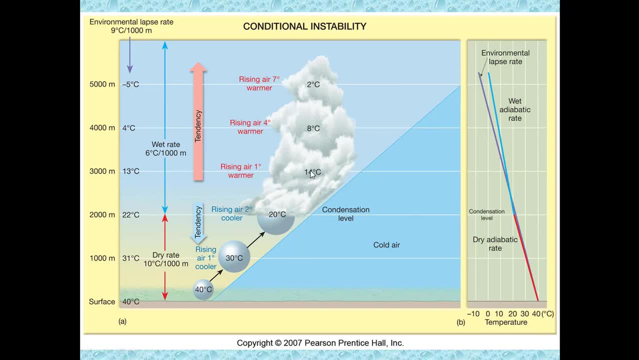 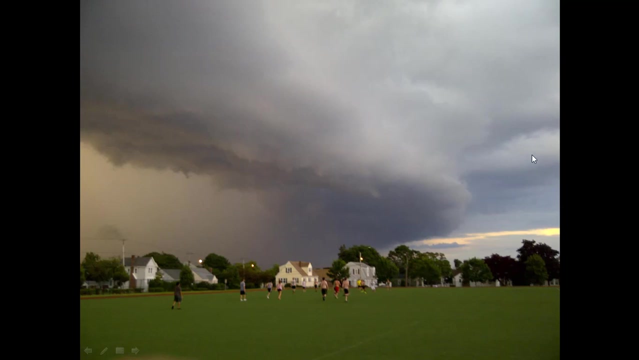 it was warmer than its overall environment and therefore now became unstable and just kept rising in the atmosphere. so that's what a conditional instability atmosphere type is, and oftentimes it can create some really intense thunderstorms. 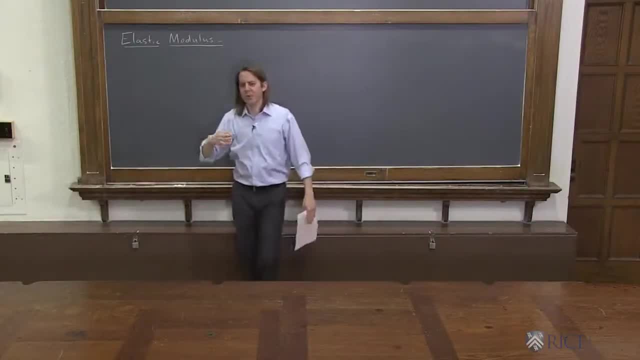 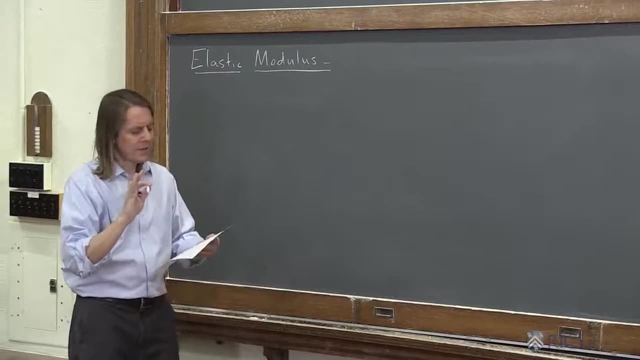 Our next topic is the elastic modulus. So before we get into a bunch of demos and problems and specifics, I wanted to give you a couple of general things about what this means. So one is, if you think back, we started with point masses. 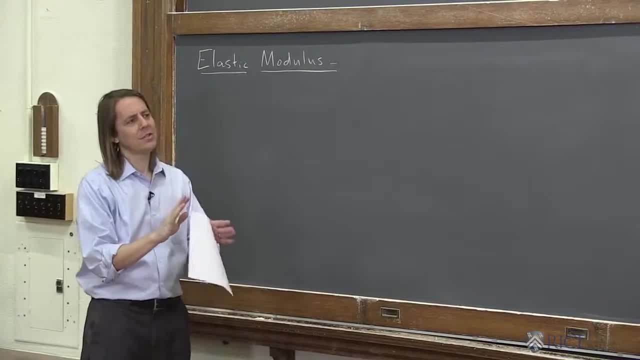 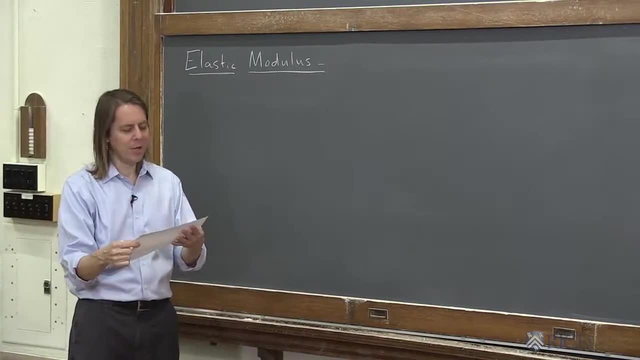 and we did forces on point masses, kinematics, And then we said, well, actually let's think about extended objects. And then suddenly their direction mattered And we did rotations and torques and angular momentum. So now we're taking it one step further. 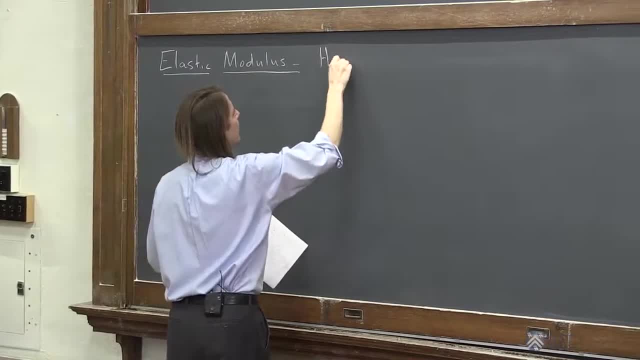 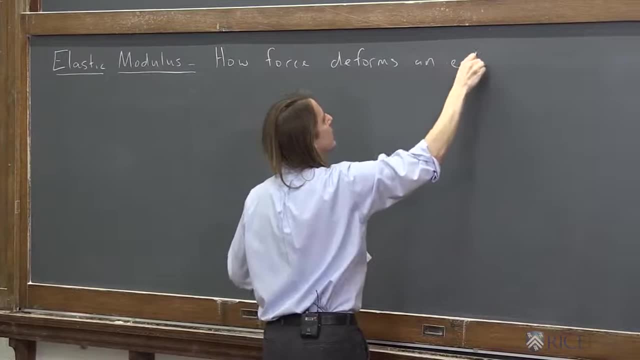 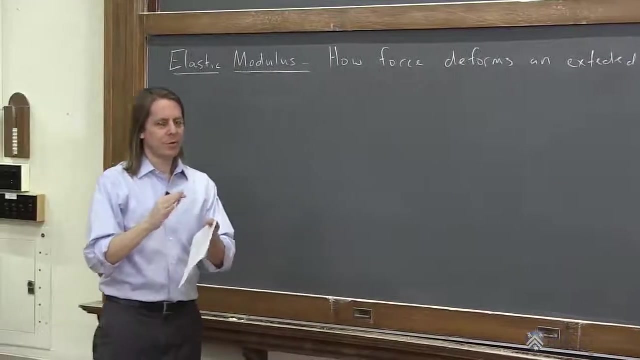 We have extended objects, but the elastic modulus is about how force deforms an extended object. So it's not really about the kinematics or the motion of the object, It's about the deformation of the object. The other thing I wanted to point out: 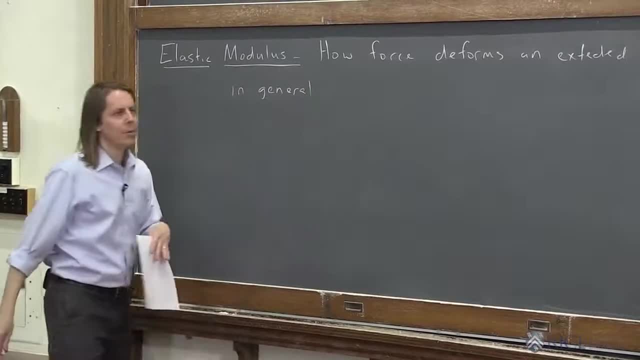 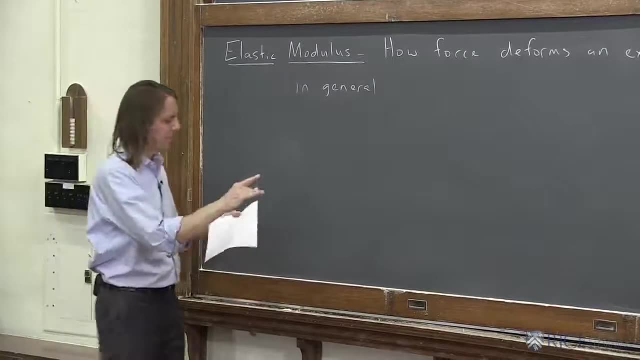 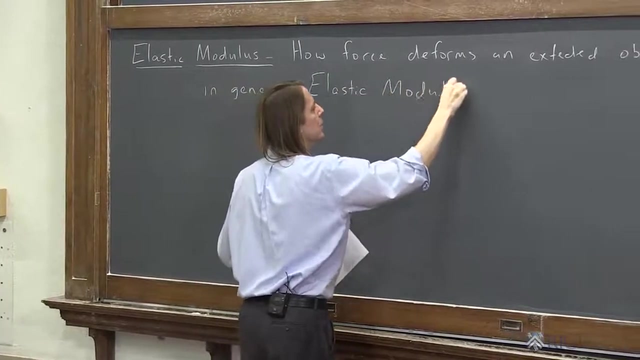 is that there are many elastic moduluses or moduli, But I want to show you how they're all really the same. So there are lots of definitions. I'm going to show you three of them, But in general, the elastic modulus, an elastic modulus. 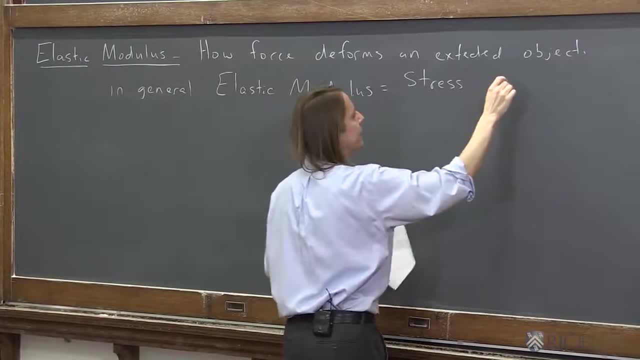 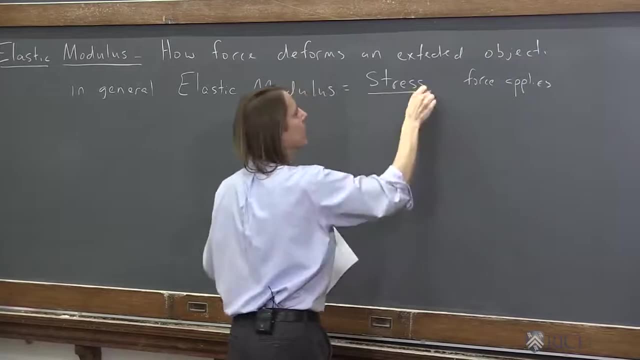 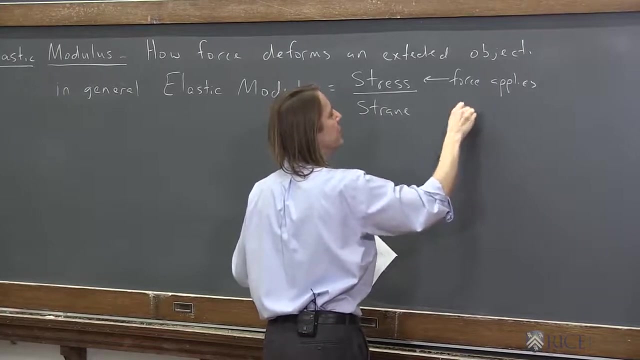 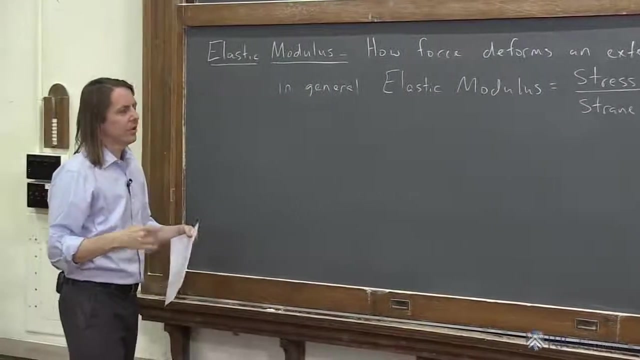 equals some stress. That's the force applied. That's some version of the force, some version of the force over the strain, And that is sort of the mechanical. the deformation is the strain right there. So now we're going to look at several versions.